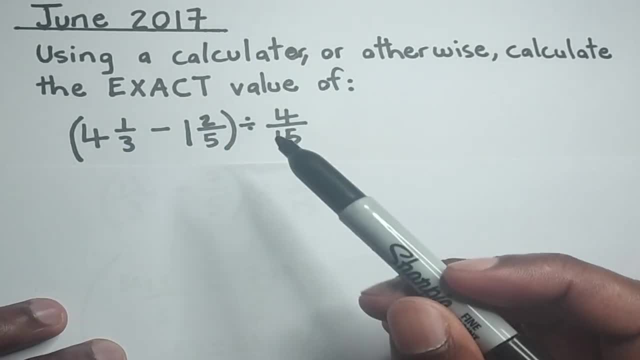 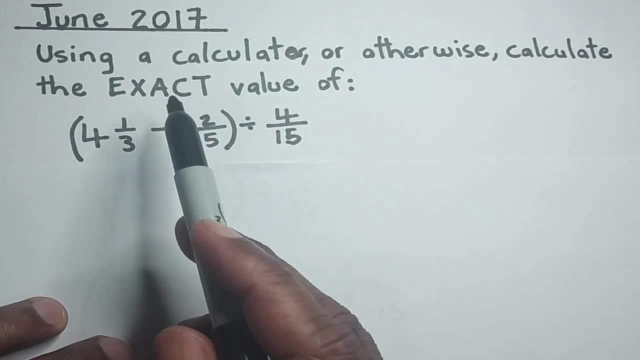 question on the June 2017 paper, and this asks us to use a calculator or otherwise to calculate the exact value of 4 and 1 over 3 minus 1 and 2 over 5 in bracket, divided by 4 over 15 all. 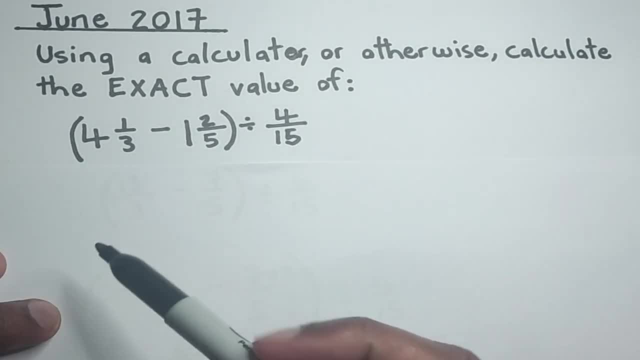 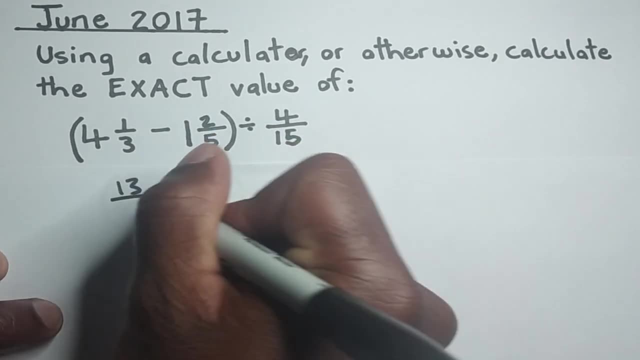 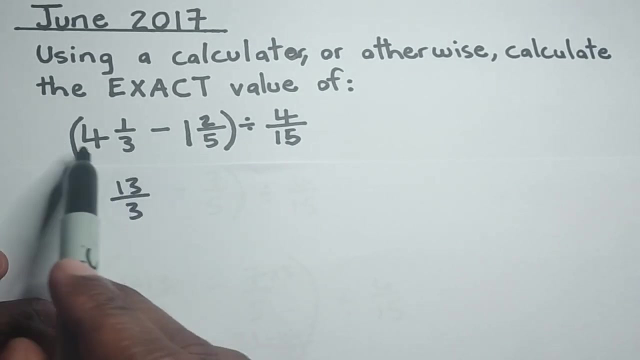 right. So what we're going to do first is to convert the mixed fractions to improper fractions. so that's what we're going to do. So 4 over 3 is the same thing as 13 over 3, and if you're not comfortable with fractions, then what I simply did- we actually multiplied the whole number by the. 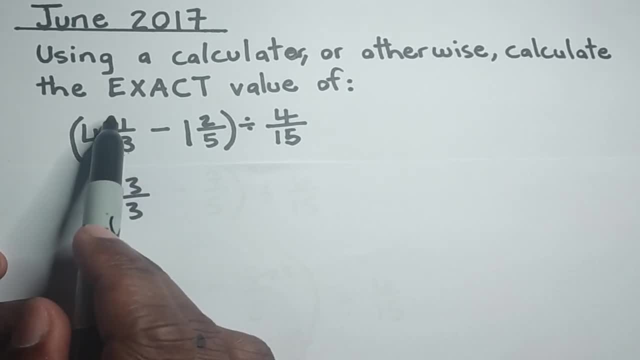 denominator, So 4 times 3.. That's 12 plus. and then we add the result to the numerator right here, so 4 times 3, that's 12 plus 1, that's 13. all right, and we kept the denominator right there, so 13 over 3 minus. 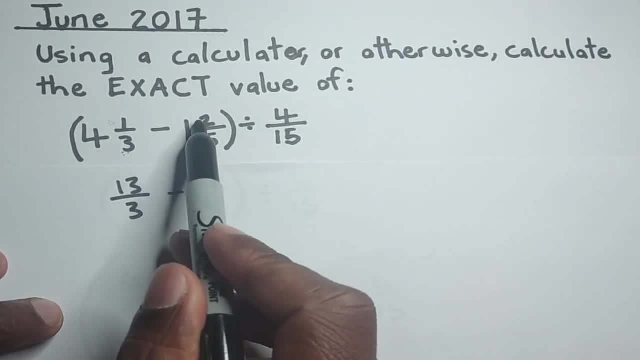 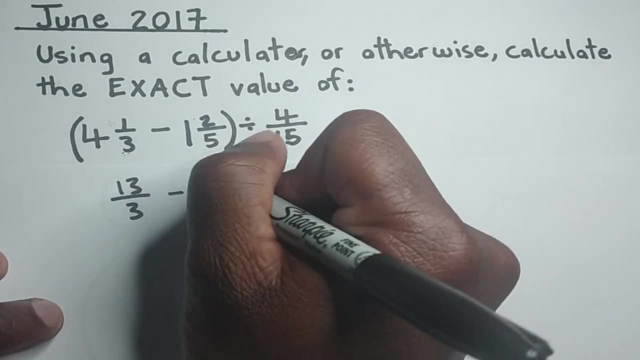 and again we do the same thing. 1 times 5, that's 5, and then we add the result that we got to the numerator. so 1 times 5, that's 5 plus 2, that's 7 over 5. all right, Now what we are going to do. 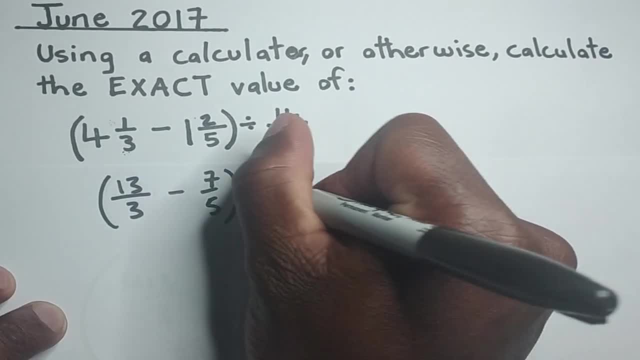 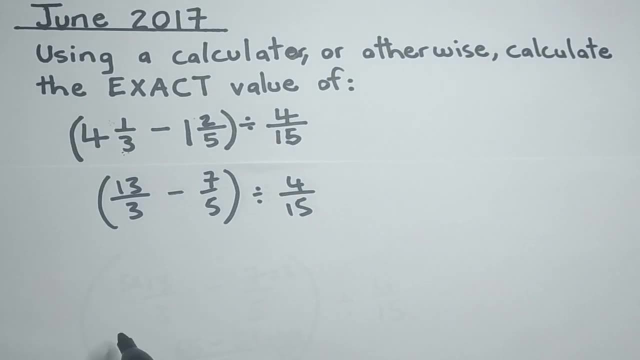 now remember we had this in bracket, can't forget about that. and we have 4 over 15, all right. What we are going to do now is to simplify what's in the bracket. now we can subtract these fractions, and what we're going to do, the method I'm going to use, 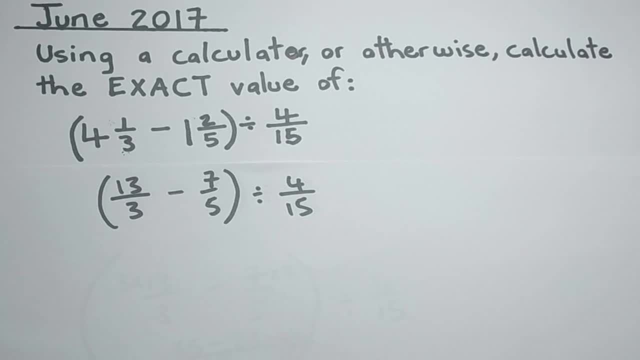 all right, might be new to you, but it's very easy, especially if you're not comfortable with LCM. So what we're going to do if we have 5 in the denominator over here, we're going to multiply this by 5 over 5. all right, so look at what i'm going to do here. i have the 13 over 3 minus 7 over 5. 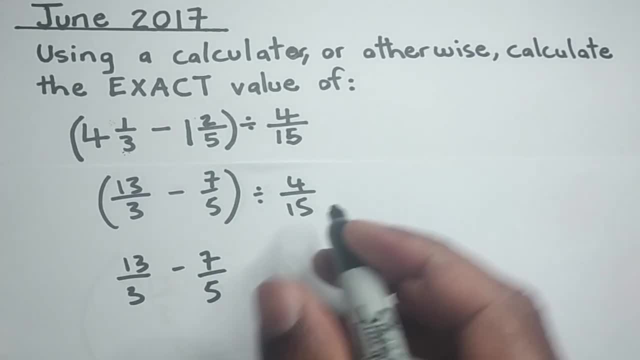 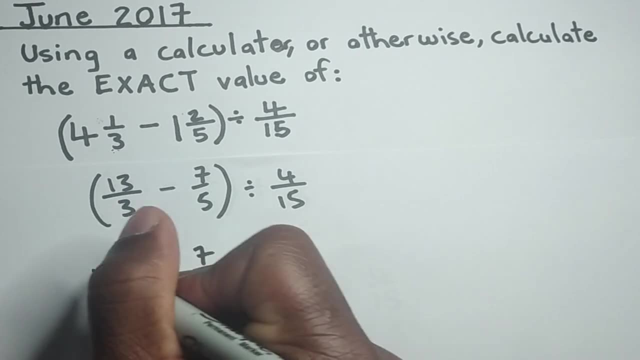 and i'm just looking at the bracket now. all right, we won't forget about this guy over here. we'll come to him sooner or later, all right. so what we're going to do if we have 5 over here? we're going to multiply over here by 5, over 5, all right, and we're doing this to obtain common. 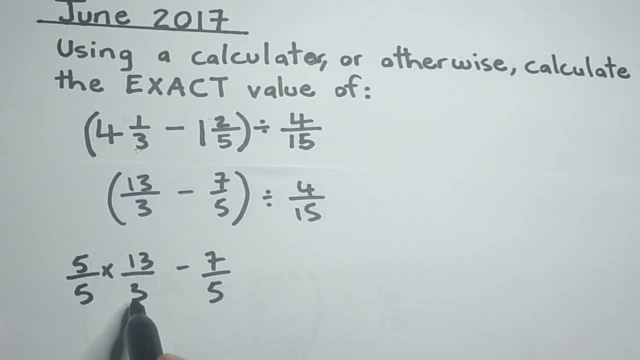 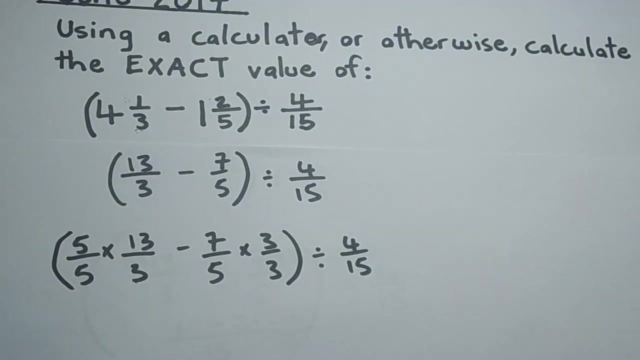 denominators. all right, and if we have 3 in this denominator, we are going to multiply over here by 3 over 3. all right, let's see what happens when we do that. so we are going to keep this thing in bracket divide. remember this thing. we are dividing by 4 over 15. now we have 5 times 13. that gives me. 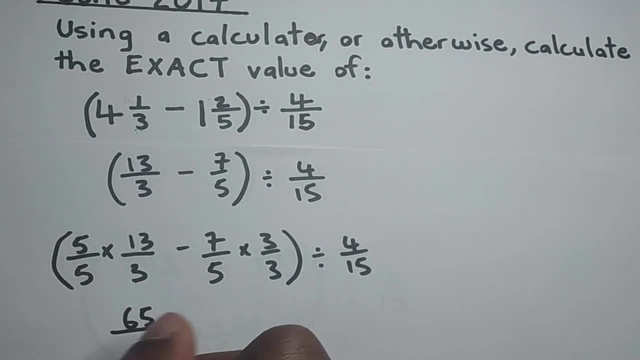 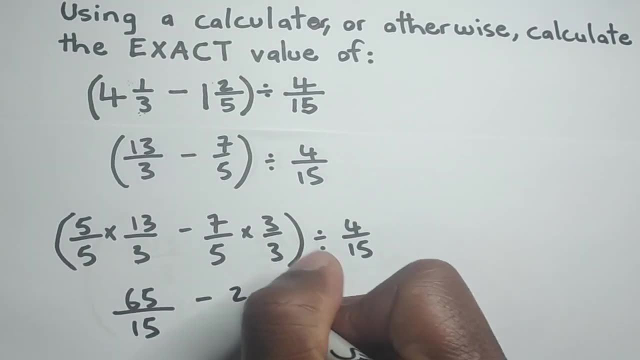 65 over 5 times 3, which is 15 minus 7 times 3. that's what 17, 17, 5 times 3 is 21. over 5 times 3 is 15. all right, now we have common denominators. so that's what we're working towards: once we can, once we have common denominators, we can. then 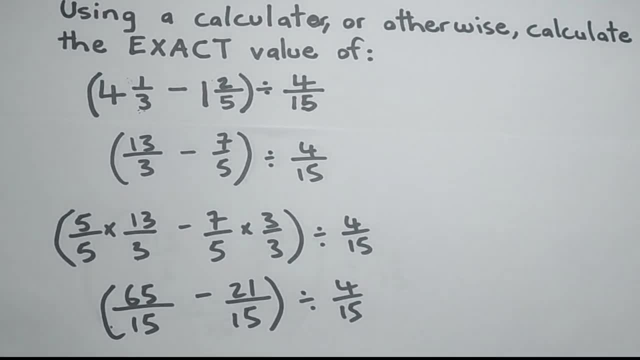 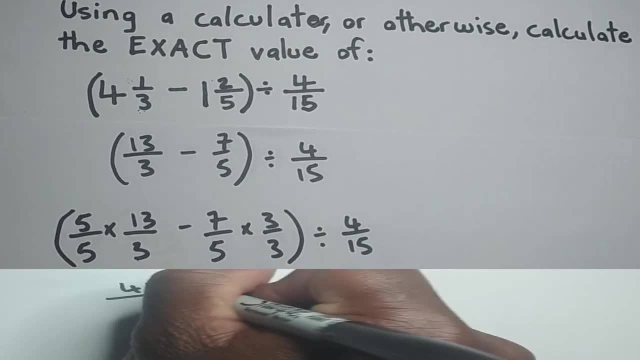 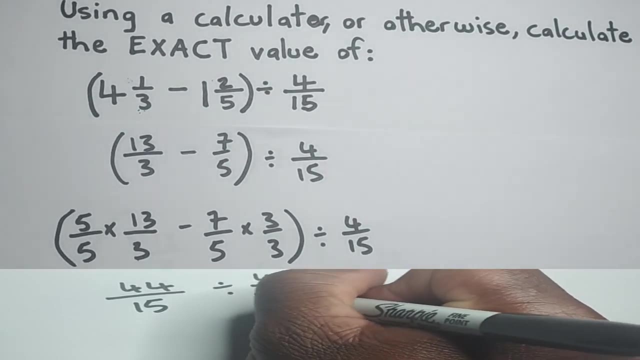 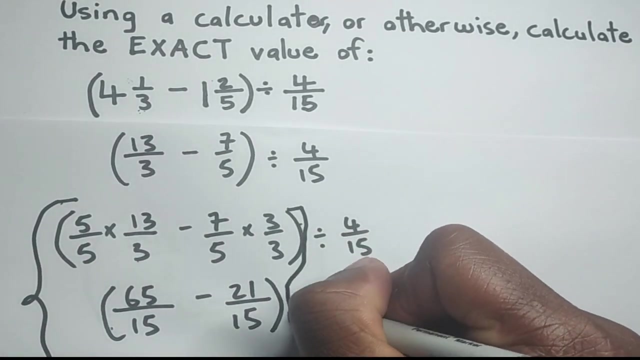 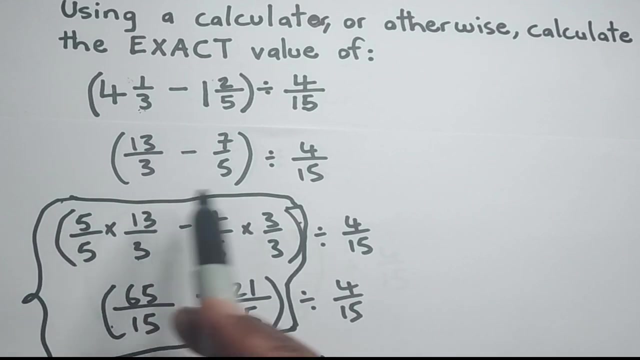 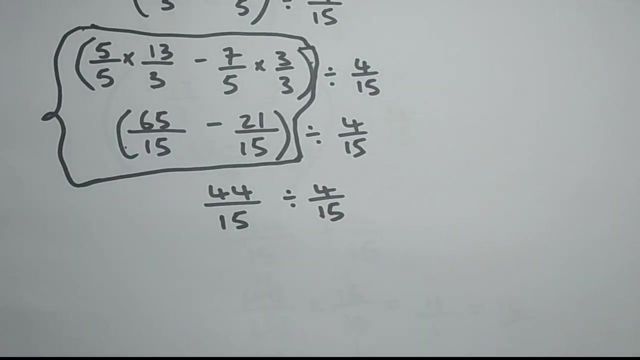 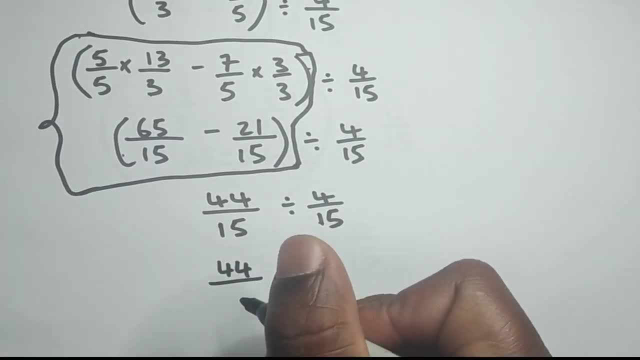 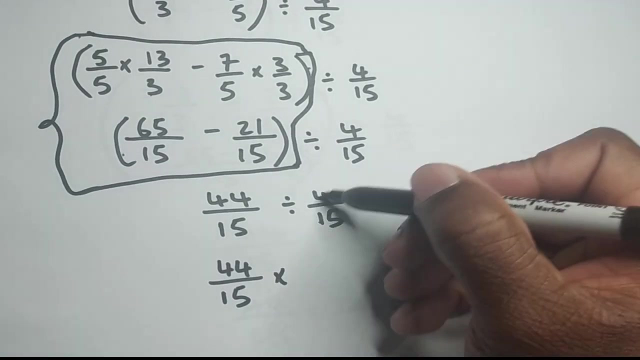 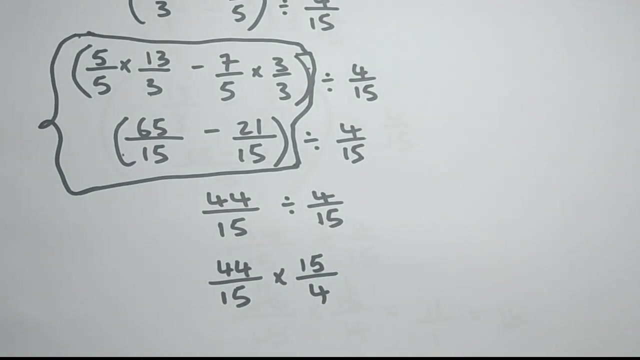 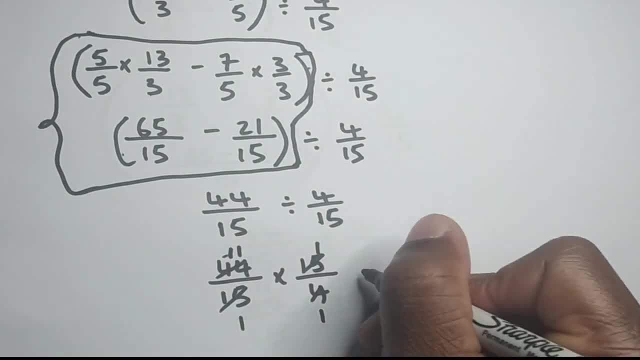 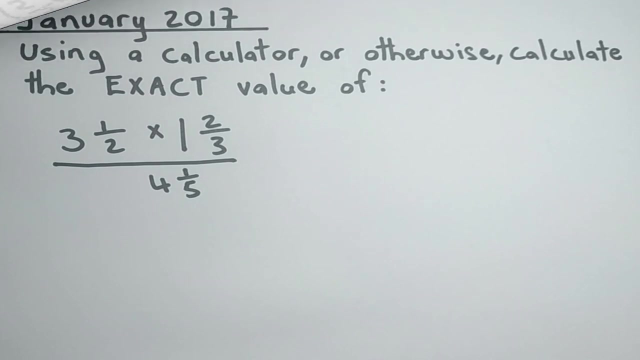 into four, one time four into forty four goes eleven. ten eleven times one, that's eleven one times one is one, and eleven divided by one will remain eleven. all right, so that's how we go about solving that question. now, here we have january 2017, all right, and this was a fraction question. 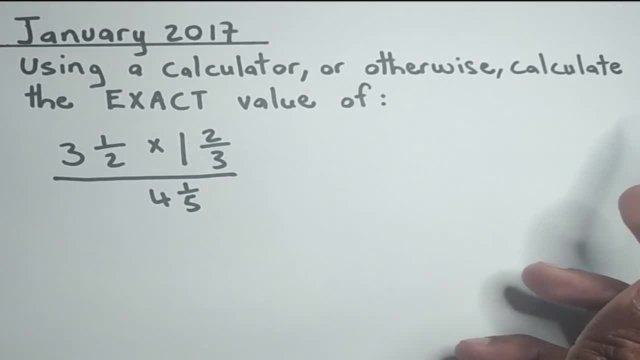 on the paper. so, using a calculator or otherwise, calculate the exact value of three and one over two times one and two over three, all over four and one over five. all right now, the thing i always tell my students to do. if you're not comfortable working fractions, that looks like this: you can. 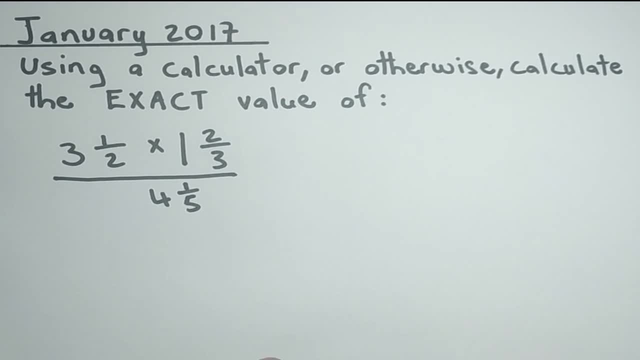 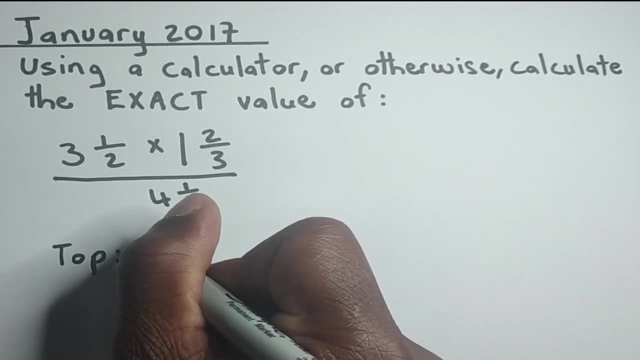 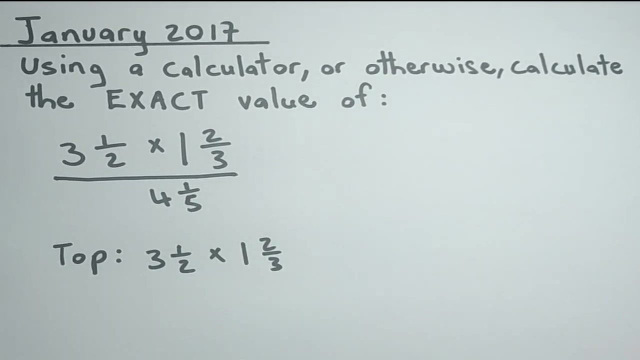 always separate the numerator from the denominator, all right? or, if you're comfortable, we can call the numerator top. so we have top and we write out what's in the top. so we have three and one over two times one and two over three. all right, so the first thing that we want to do again is to convert the mixed fractions into improper. 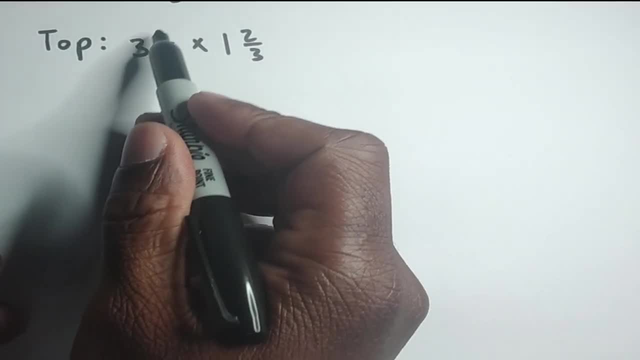 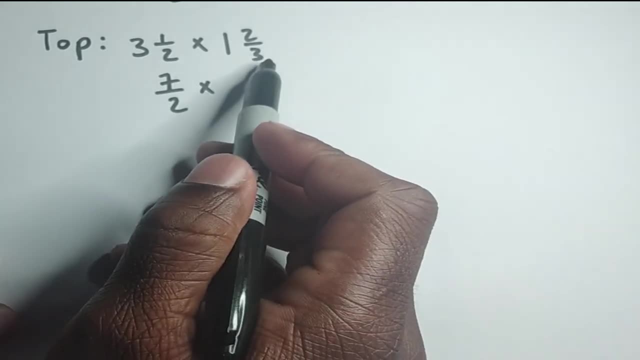 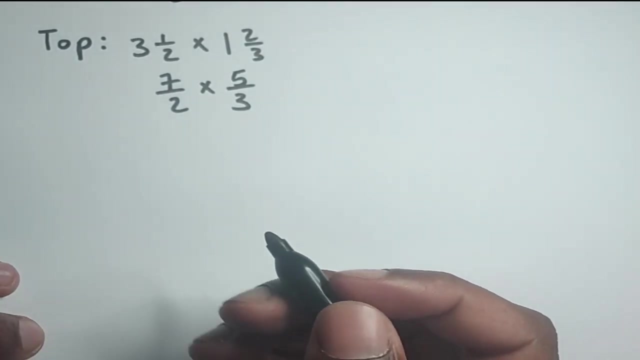 fractions. all right, so we'll have three times two, that's six plus one, that's seven over two. times one times three, that's three plus two, that's five over three. all right, where can we go from here? now we can multiply the numerator: times numerator denominator. times denominator. 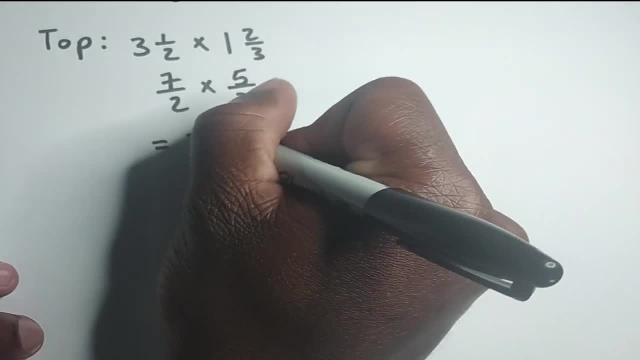 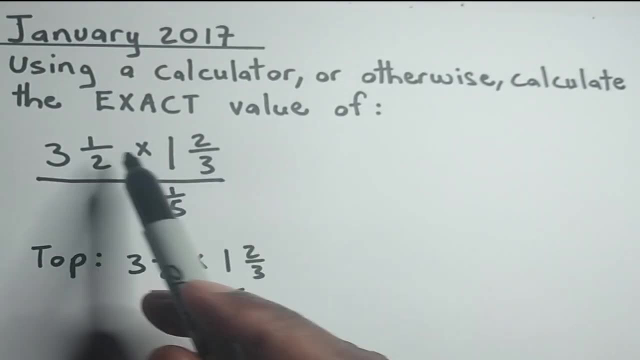 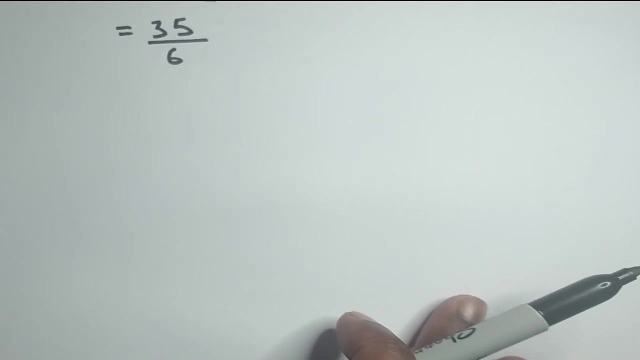 so seven times five, that's thirty five over two times three, that's six. all right, so when we work out the numerator here, which is three and one over two times one and two over three, we'll obtain the value of 35 divided by six. all right, so that's what we'll get. now we want to start the denominator. 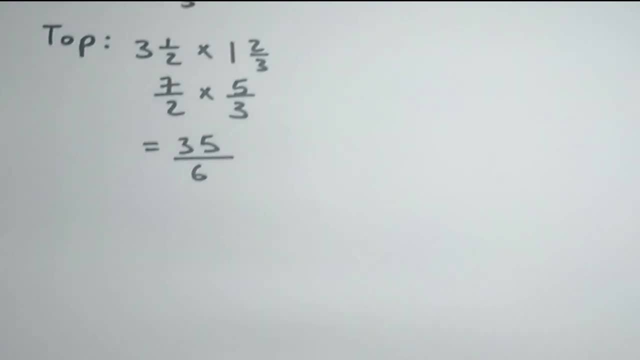 all right, so we have four and one over five. so we're going to convert the four and one over five to an improper fraction. so we're going to convert the four and one over five to an improper fraction option. all right, so let's convert this thing now. so we have four. this is what we have in the 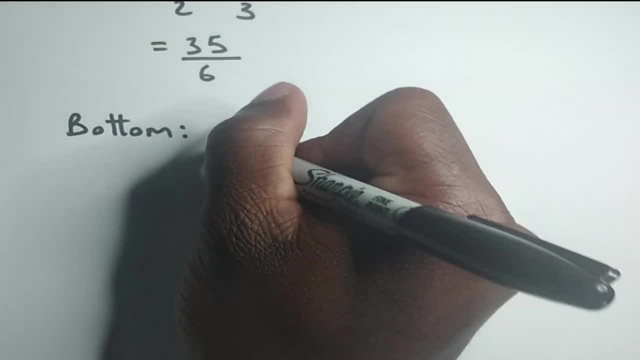 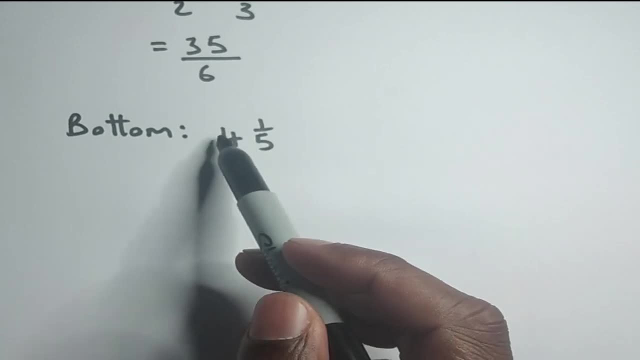 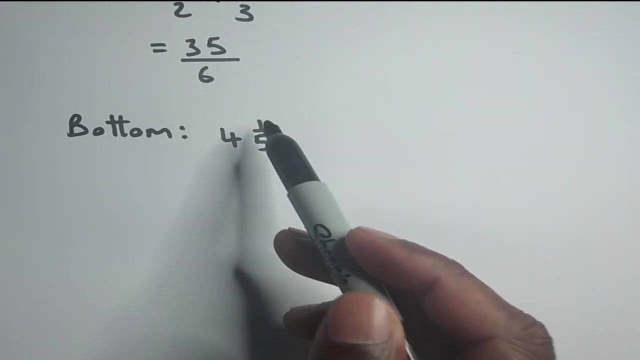 denominator. so we have four and one over five. so how do we go about this? again, we'll multiply the whole number by the denominator, then add the numerator. all right, so we have four times five, that's 20 plus one, that's 21. so this is the same thing as 21 over the denominator, which is five. 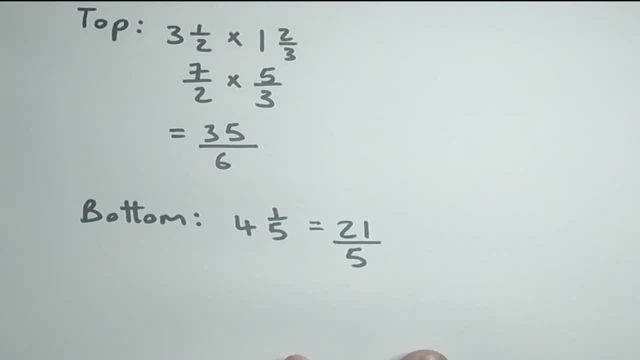 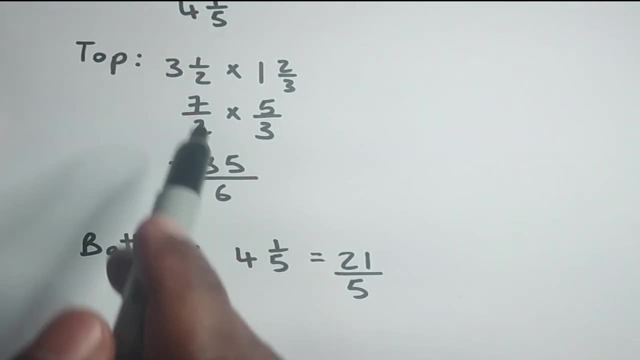 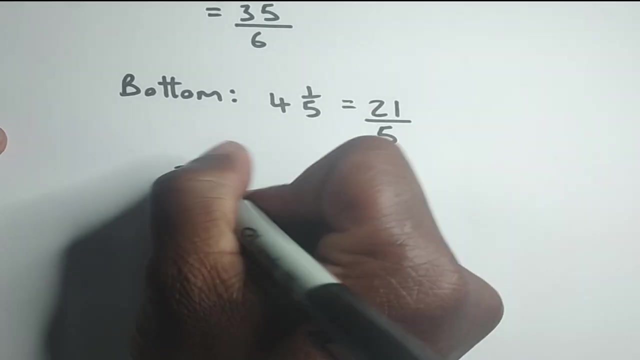 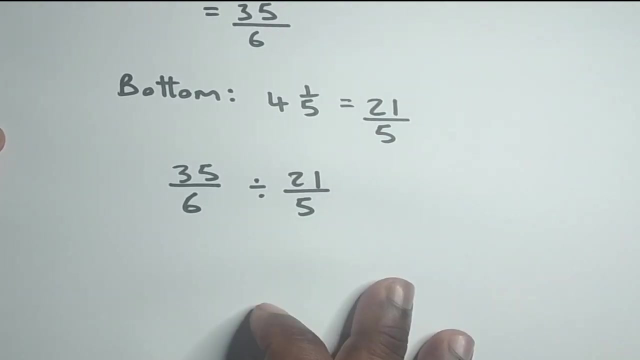 all right. so that's how we treat with that now. what we're going to do now is to divide the numerator by the denominator, all right, or the top by the bottom. so here we would have 35 over 6 divided by 21 over five, all right. so again remember, when we're dividing fractions, we keep the first fraction. 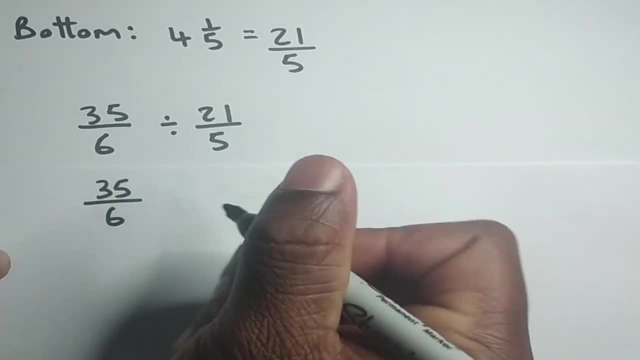 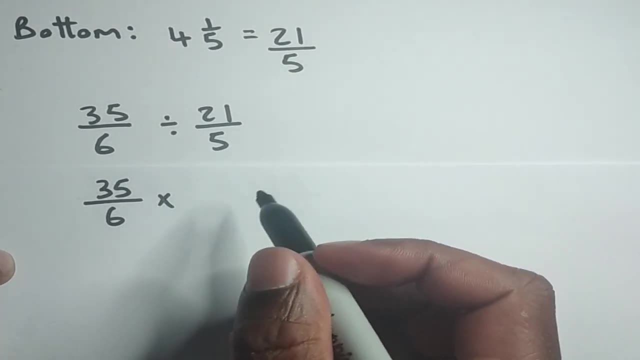 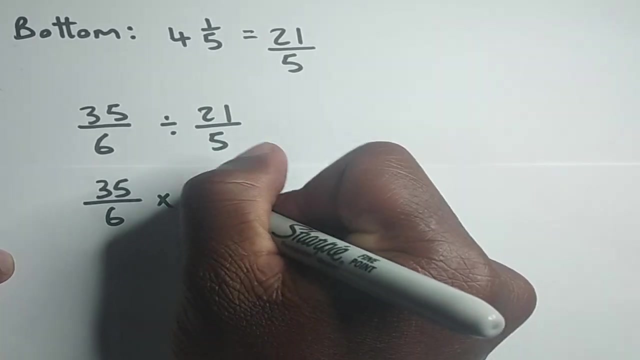 which is 35 over six. then we change the division sign to multiplication and then we flip the second fraction. all right, so i will reciprocate the second fraction, so that simply means 21 over five will become five over 21, all right, and we can simplify this thing so. 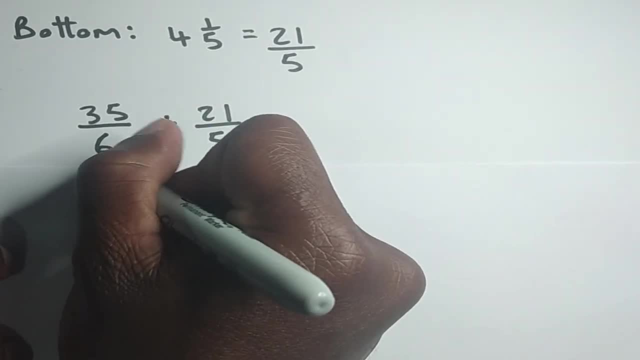 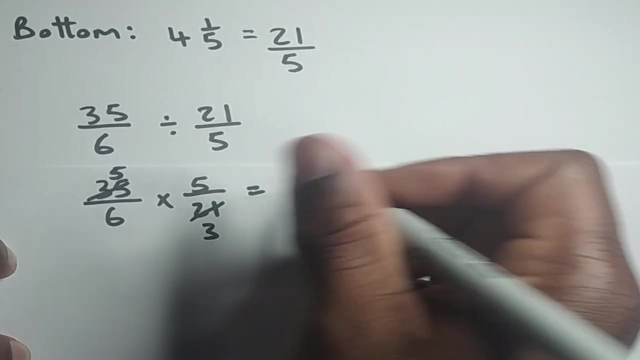 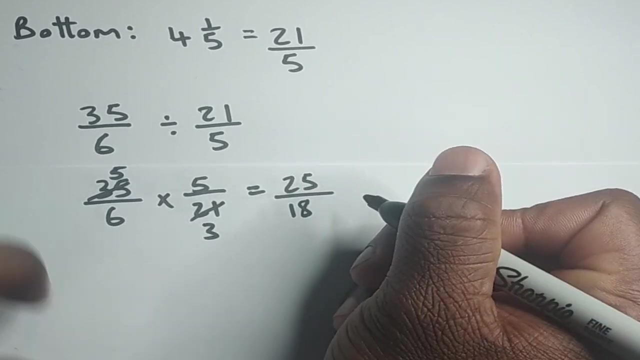 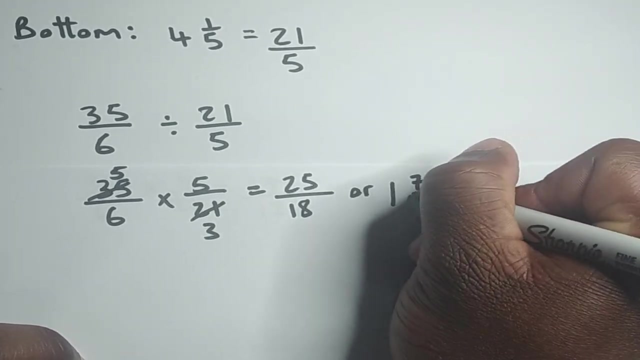 seven can go into 35 five times, and seven can go into 21 three times, all right. and then now we can multiply across, so five times five, that's 25 over six times three, which is 18, all right. and we can also write this in mixed fraction, also: 18 going to 25 one time, with a remainder of 7. 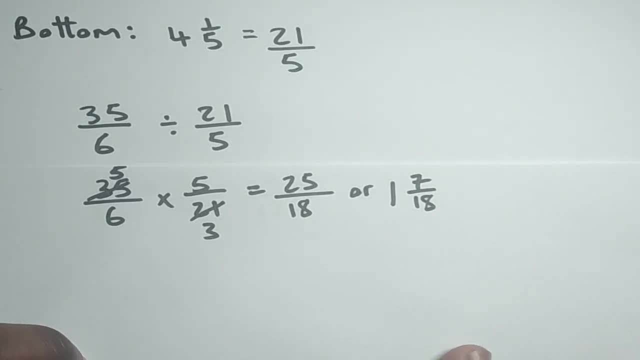 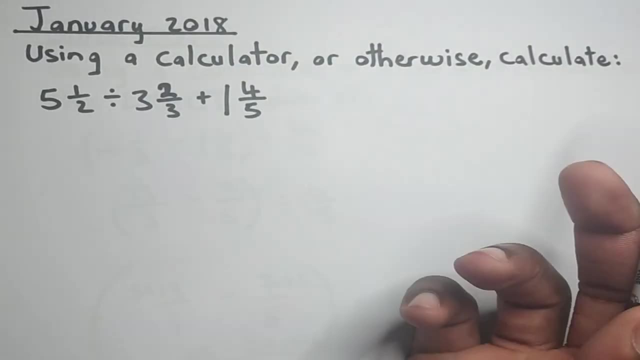 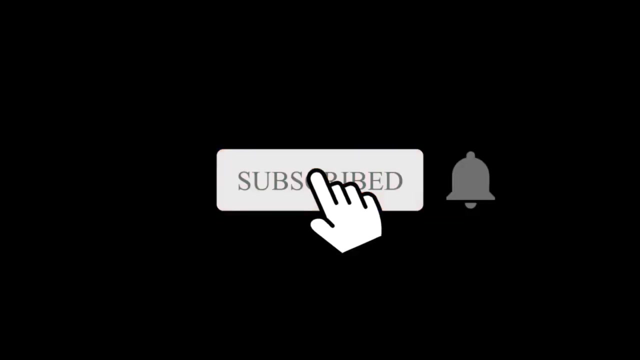 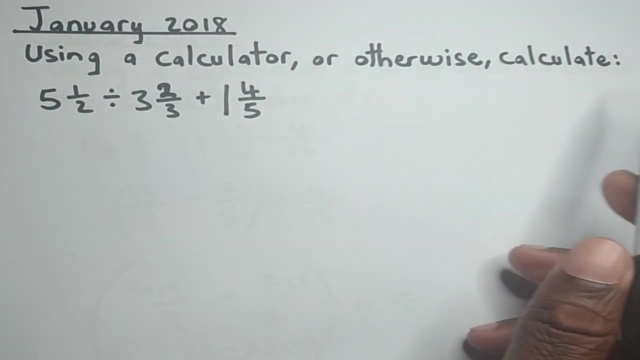 over 18. all right, so that's pretty much how we treat with this question. now we are looking at january 2018 and this was the fraction question on this paper, right? so this asks us, using a calculator or otherwise, calculate five and one over two. 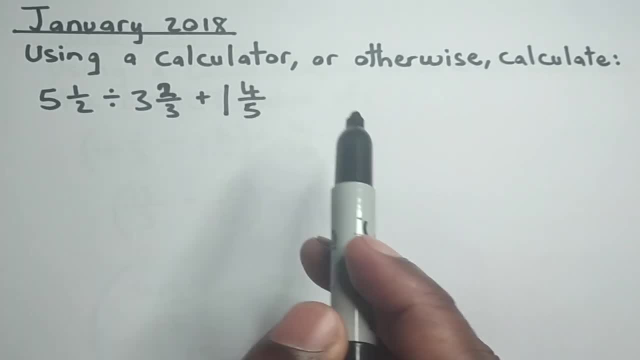 divided by three and two over three, plus one and four over five. all right, so according to the law of operation, we are going to calculate five and one over two, divided by three and two over three. operation or order of operations. rather, we are required to divide first before we can. 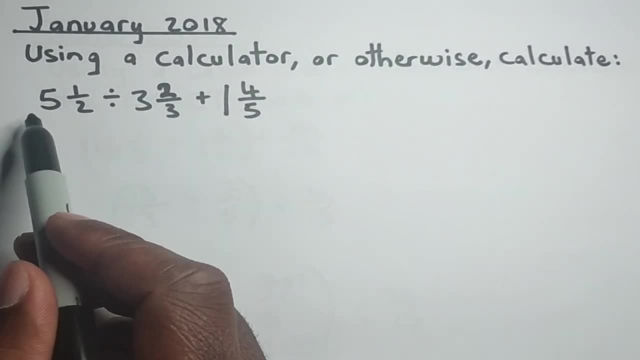 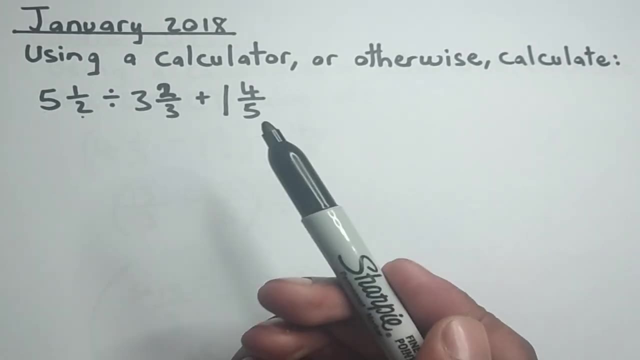 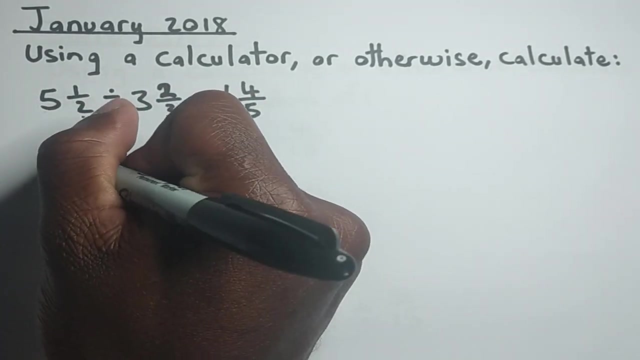 add. all right. but what we are going to do first is to convert all the mixed fractions to improper fractions, all right. and again we multiply the whole number by denominator, then add the product to the numerator. so five times two, that's ten plus one, that's 11. so five and one. 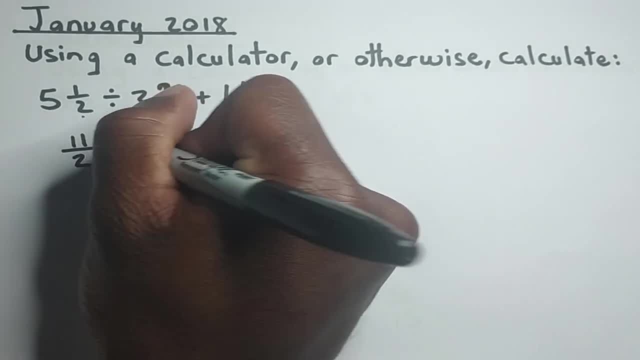 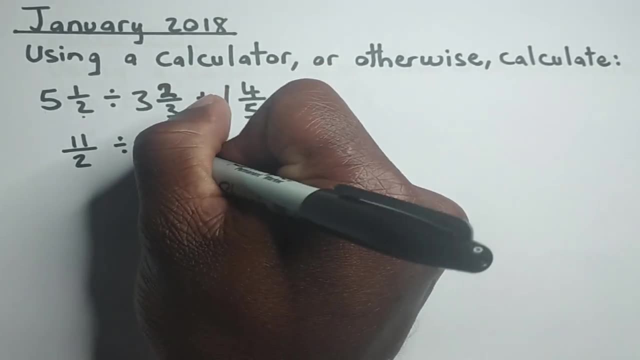 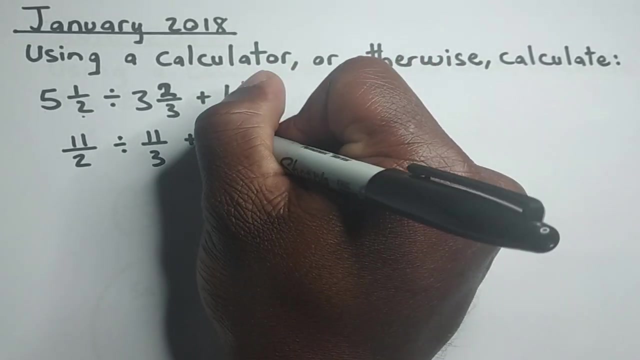 over two is the same thing as 11 over two. divided by here, we have 3 times 3, that's 9 plus 2. this is also 11 over 3 plus here we'd have now 1 times 5, that's 5 plus 4, that's 9 over 5. all right now when we're dividing again, so we could. 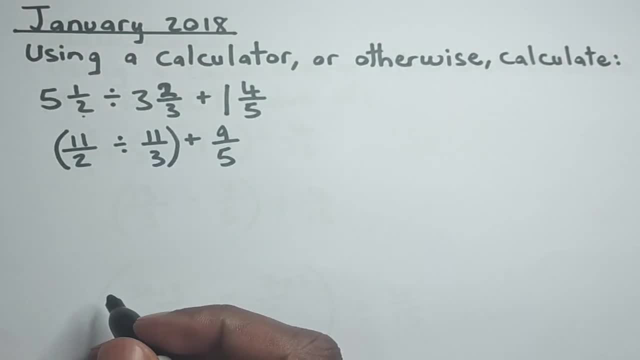 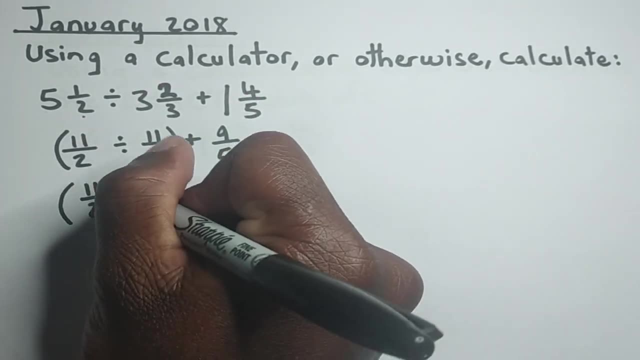 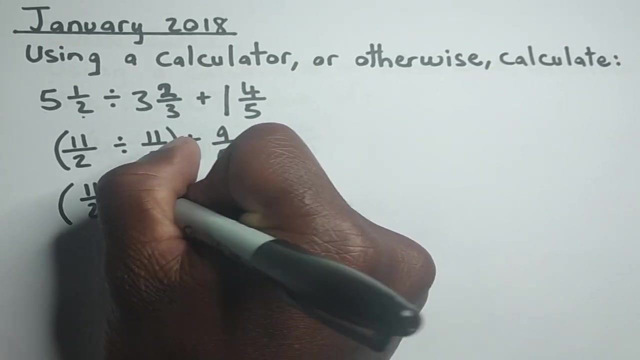 put this thing in bracket, because we have to divide first. all right. when we're dividing now, we are required to keep the first fraction, so always remember that. then we do a change, a division sign to multiplication. then flip the second fraction, so 11 over 3 will become 3 over 11. 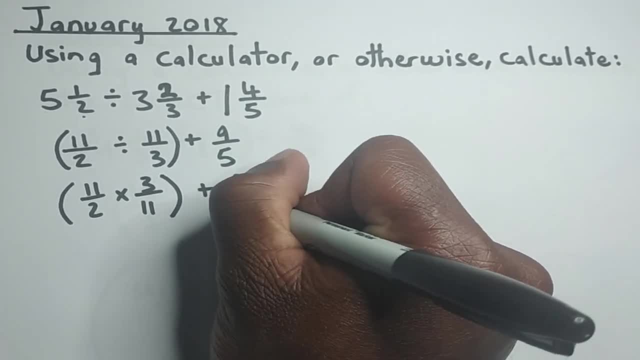 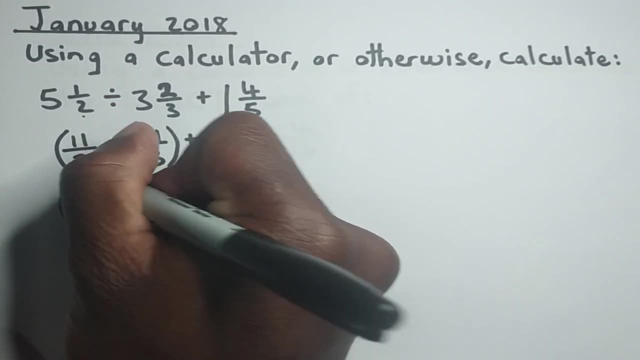 all right, and we still have to add the 9 over 5 right here. all right, we can simplify this thing. so 11 will cancel 11, so 11 going to 11 one time. 11 to 11 one time. all right, so here would be left. 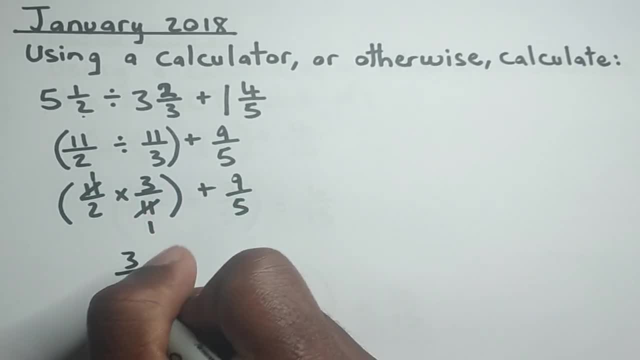 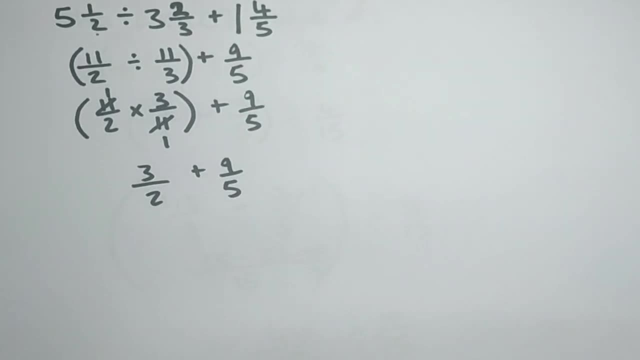 with 1 times 3, that's 3, 2 times 1, that's 2, and we're adding the second fraction. so 11 over 3 will become 3 over 11, all right, and we still have to add the 9 out here, all right. so to bring some balance to what we have done so far, I'm going 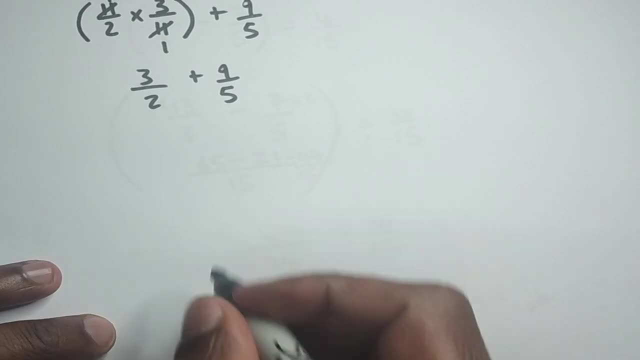 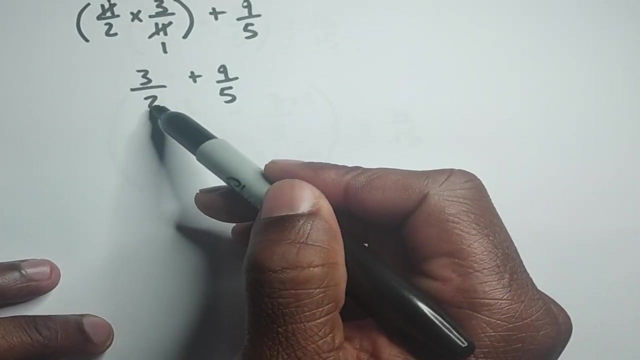 to take the LCM method to work. this one, however, you could also, being that you have 5 in the denominator over here, you could multiply over here by 5 over 5. you have 2 in the denominator over here. you can multiply over here by 2 over 2 if you so choose to, all right, but in this case, 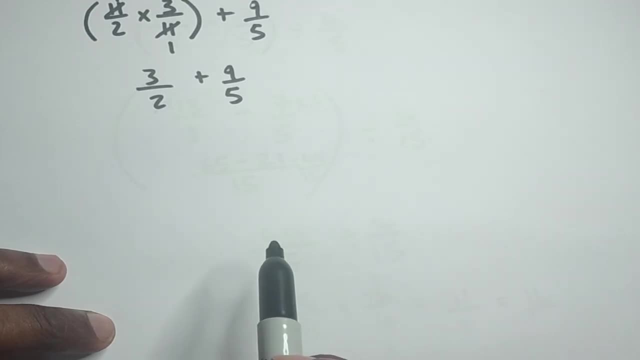 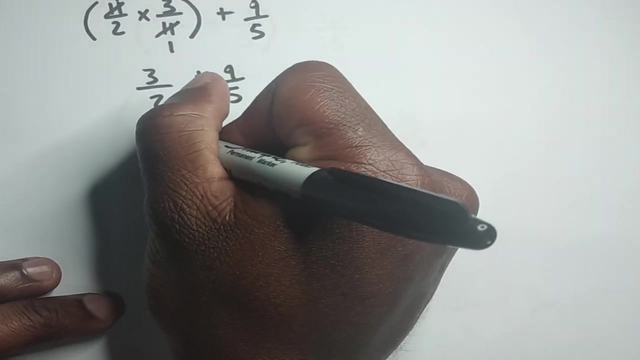 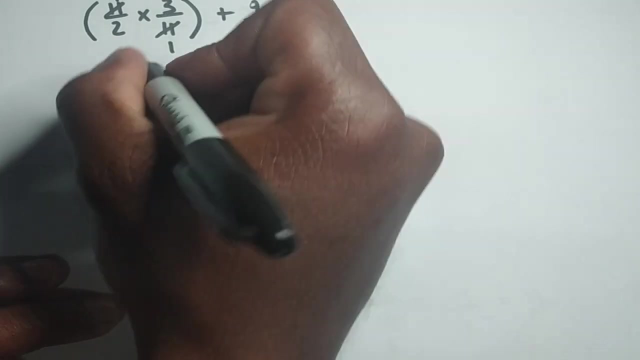 because I've done that in the previous question- then I will use the LCM method to solve this one. all right, so we're going to find the LCM. so the LCM for 2 and 5, that would be 10. all right, 2 going to 10, 5 times 5 times 3, that's 15 plus 5 into 10, that's. 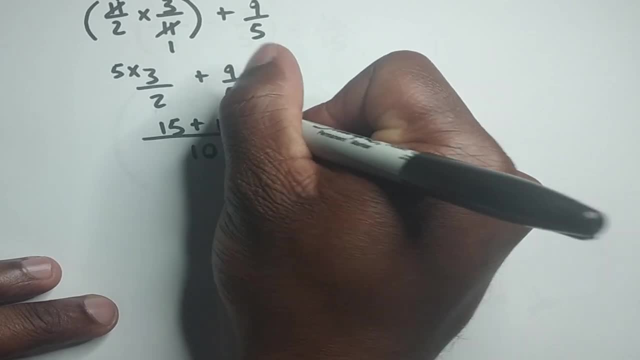 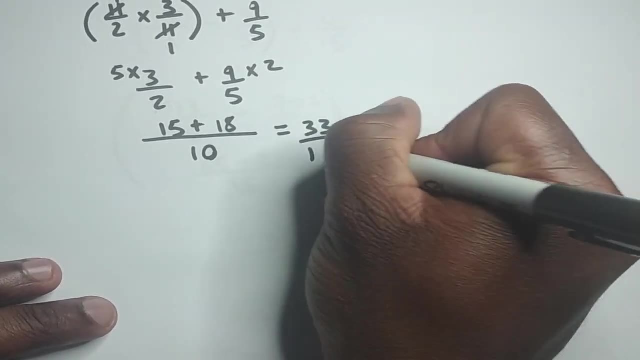 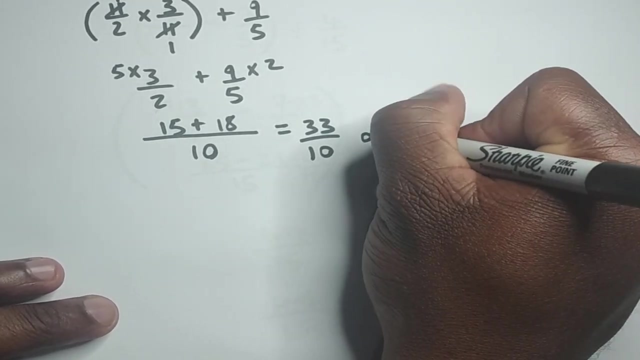 equals 2 times 2 times 9, that's 18. all right, and 15 plus 18 gives us 33, if I'm not mistaken. all right, so this would have been our solution. however, we can rewrite this thing as a mixed fraction: 10. 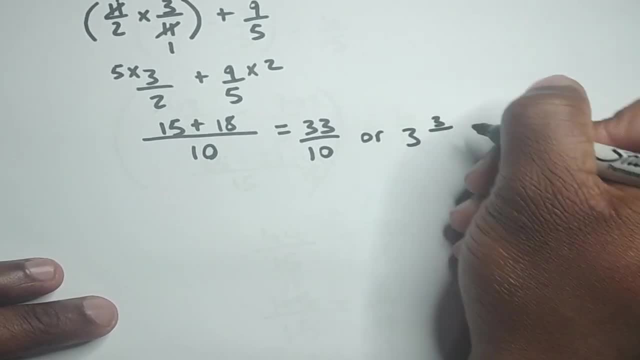 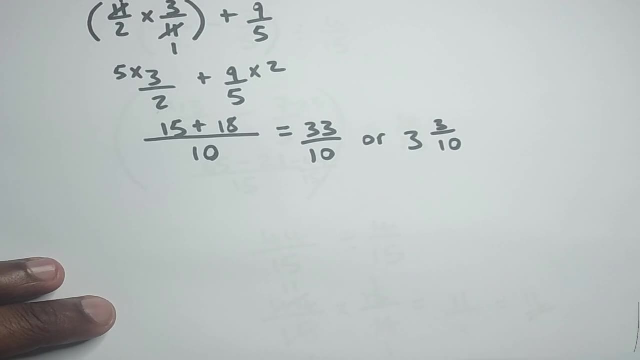 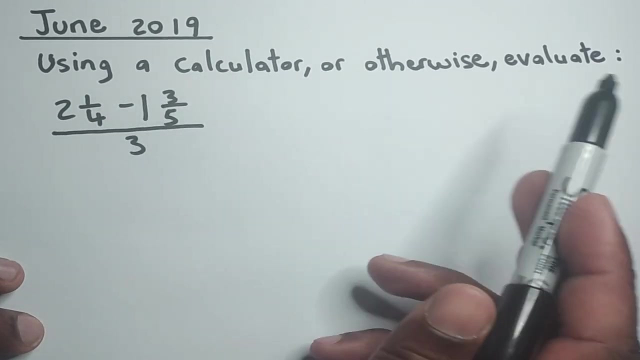 going to 33, 3 times, with a remainder of 3 over 10, all right, so this would have been our answer for this particular question. now, here we have June 2019, all right, and this asks us to use a calculator otherwise to evaluate this thing right here, which is 2 and 1 over 4 minus 1 and 3 over 5. 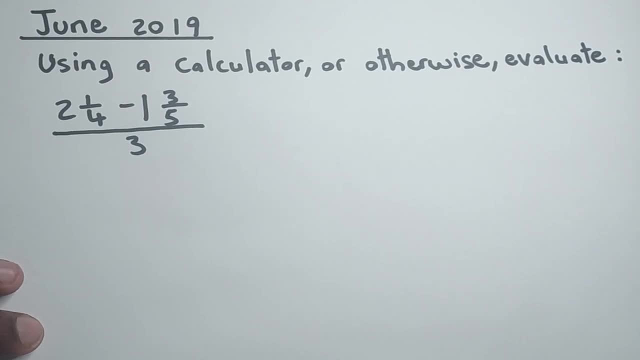 all over three. all right now. how can we go about doing this thing? all right again. as i mentioned before, we can separate the numerator from the denominator. that makes life so much easier for us. all right, so we can separate the top from the bottom. so in the top we'll have two and one over. 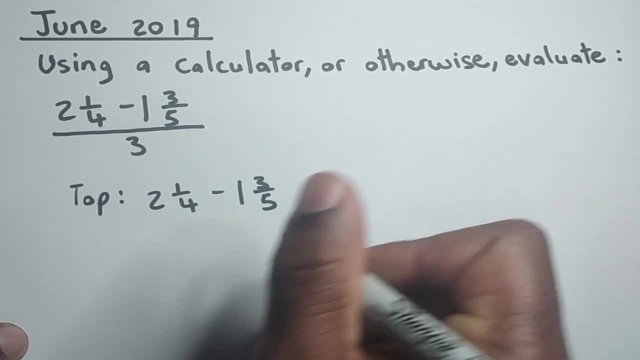 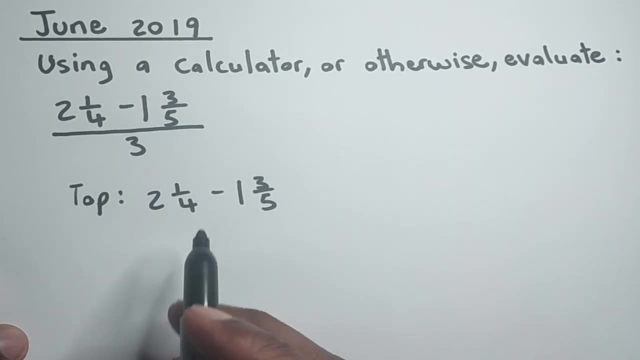 four minus one and three over five, and what we're going to do is to convert the mixed fractions to improper fractions. so we will convert this two and one over four to by multiplying the whole number by the denominator, then add the result to the numerator. so two times four is eight. 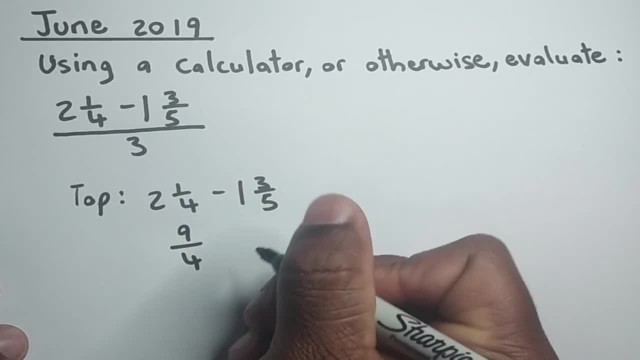 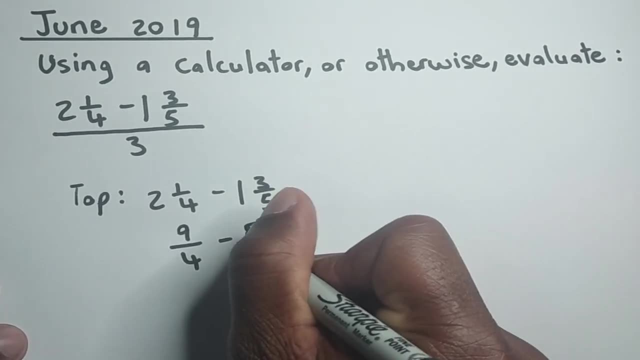 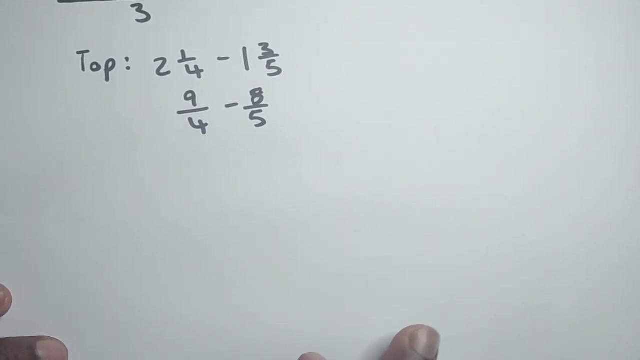 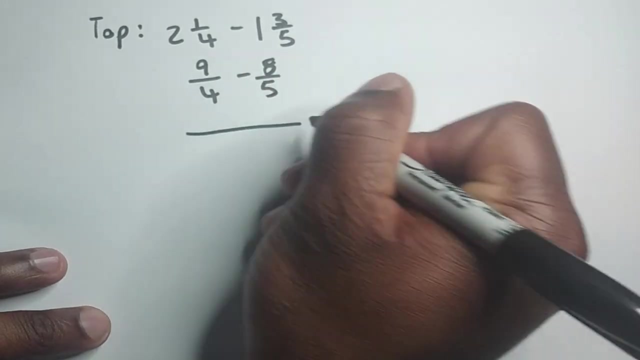 eight plus one, that's nine over four. minus one times five, that's five plus three, that's eight over five. all right, now what we're going to do? we're going to use the lca method, all right. i think most people will be comfortable with that, so i'm going to use the lca method again. so we are going to find the 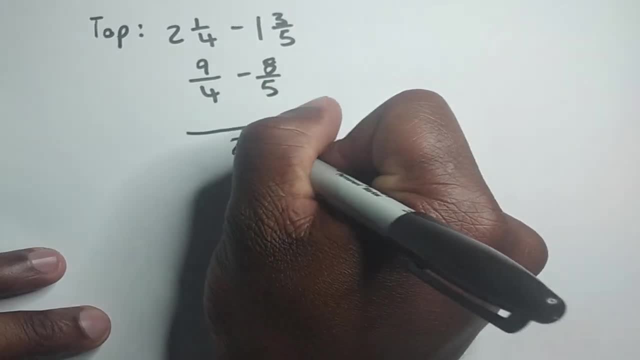 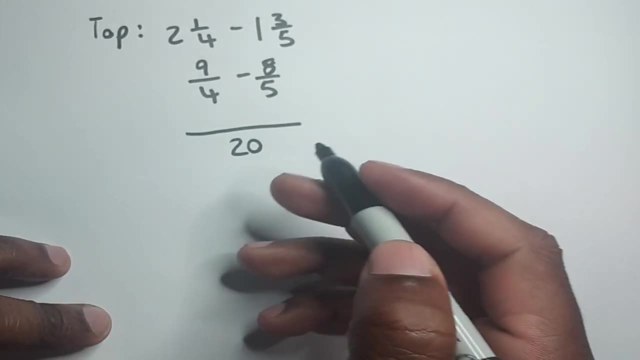 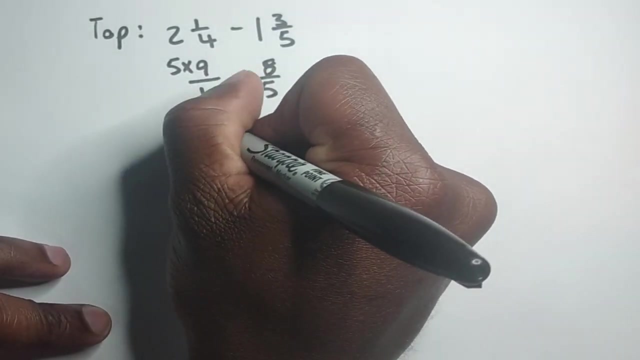 lcm for this thing, the lcm for four and five. that would be 20 again. that's the lowest number that both the denominators can go into without leaving a remainder. four into 20 goes five times. we'll multiply that by the corresponding numerator. five times nine, that's 45 minus five into 20. 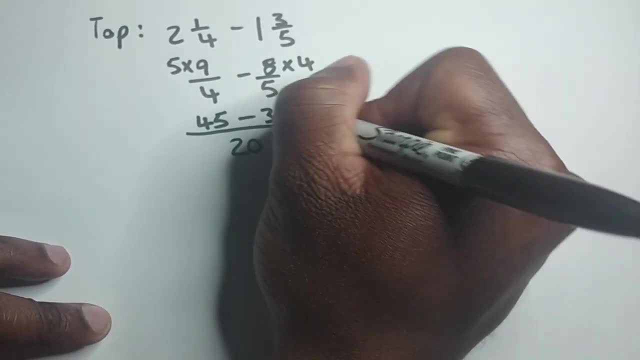 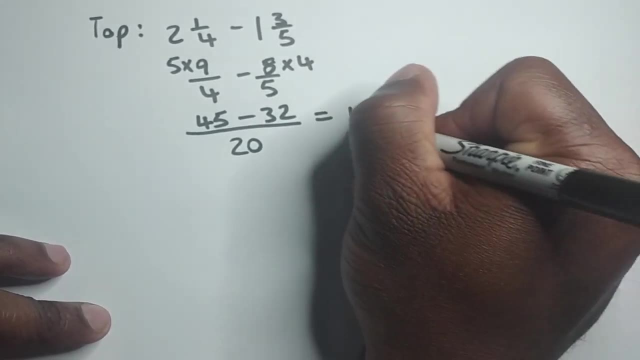 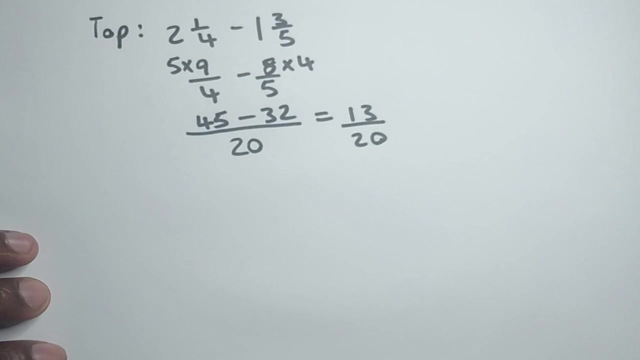 goes four times eight times four, that's 32. 45 minus 32, that's what i believe. that's 13, if i'm not mistaken. so we're left with 13 over 20 all right now, the bottom is already started. for us, that's just one. 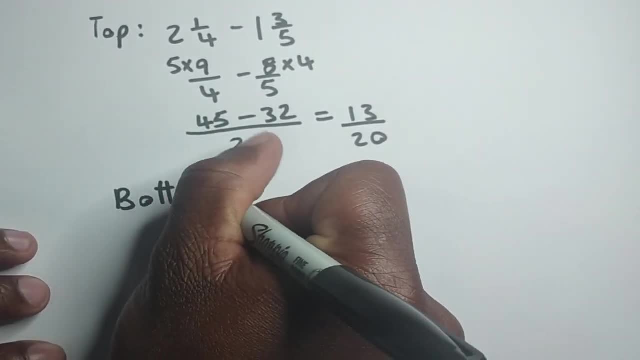 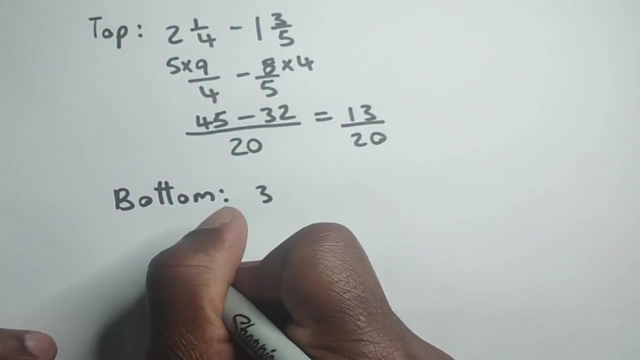 number down there. so that's three, all right. so what we're going to do is to divide the top by the denominator. so we're going to divide the top by the denominator. so we're going to divide the top by the denominator. so we're going to have 13 over 20 divided by three. all right. now a key thing to note is that 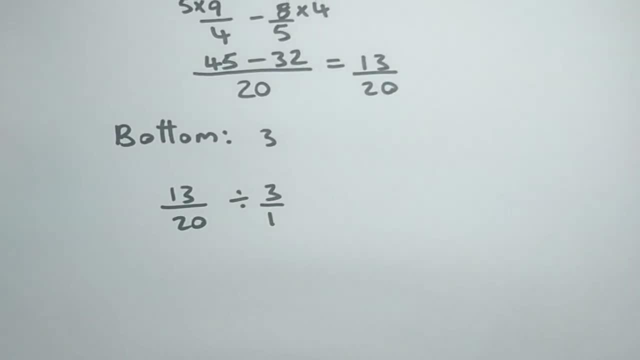 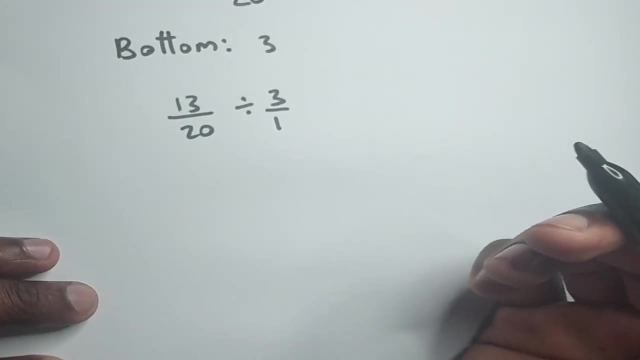 three is the same thing as three over one. all right, that's the same thing. three is the same thing as three over one, because if you divide three by one, then you'll obtain three just the same. all right, so what we're going to do again, when we divide the fractions, we keep the first. 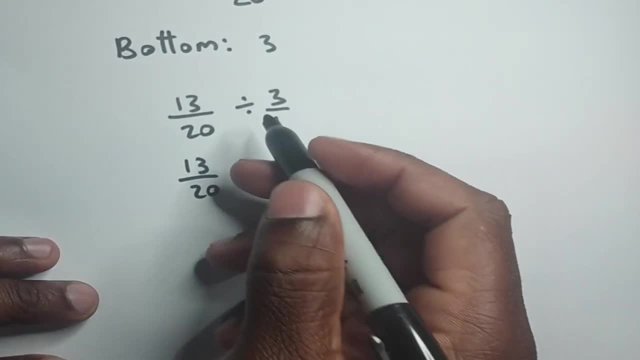 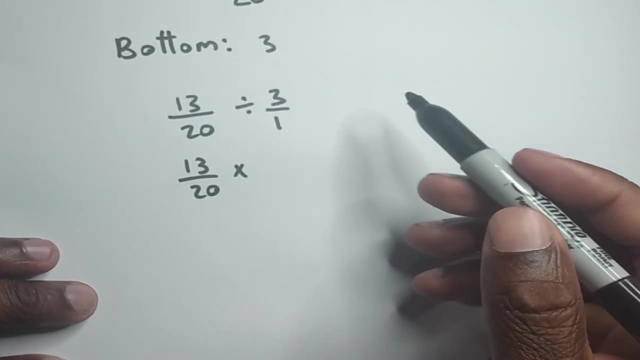 fraction which is 13 over 20. in this case, we change the dividend sign to multiple times three multiplication, then we'll flip the second fraction. all right, so that's why i did that thing, to help you better understand what will take place here. i put a place to three over one, so we'll flip. 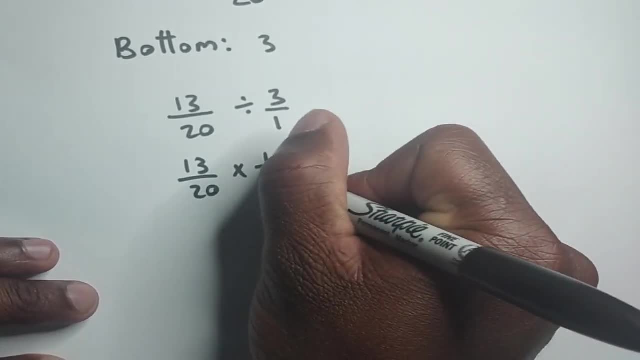 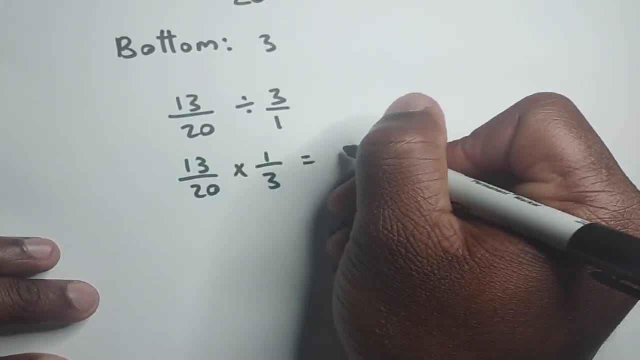 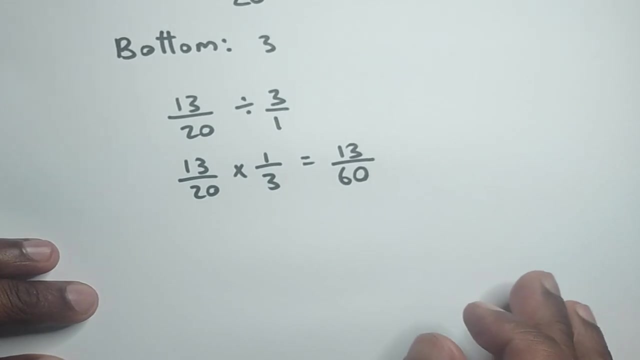 this thing. so three over one will become one over three, all right. and we can pretty much simplify this thing now. so 13 times one, that's 13. over 20 times three, that's 60, all right. so this would have been the correct answer. so we're going to do that again. so we're going to divide the top by the. 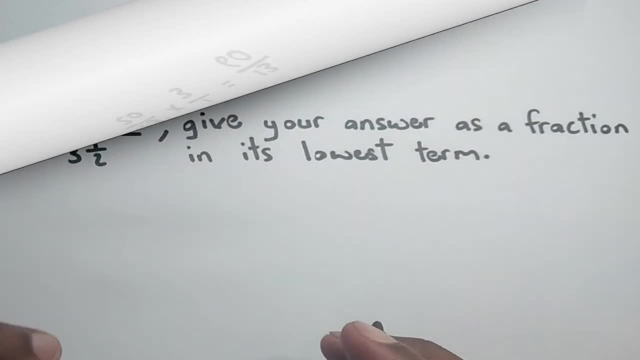 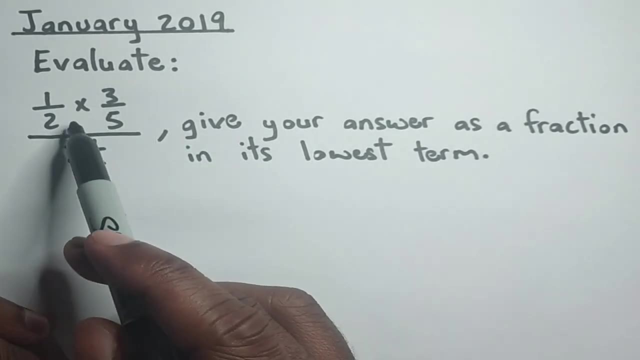 bottom. so we're going to divide the top by the bottom. so we're going to divide the top by the bottom. solution for this particular problem. now, here we have january 2019, all right. now this question asks us to evaluate one over two times, three over five, all over three and one over two. all right. 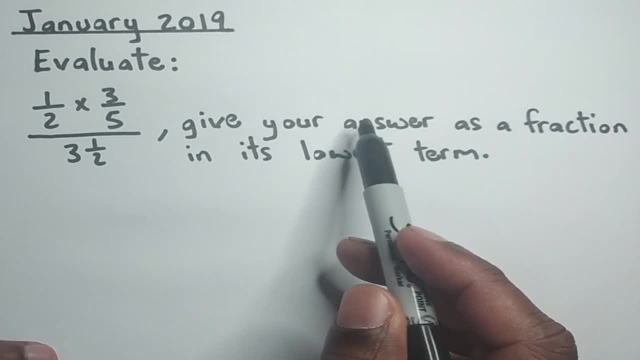 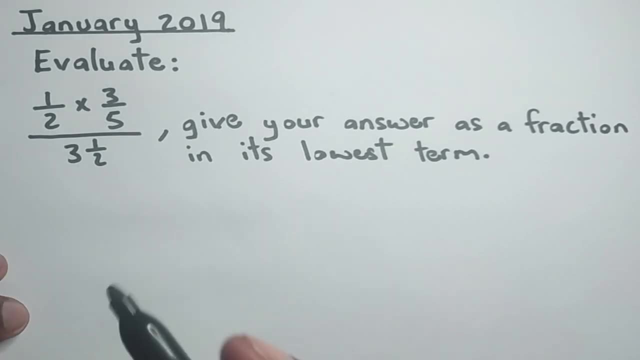 and it further going to tell us that we should give our answer as a fraction in its lowest term. all right, so we have to bear that in mind. now, again, we are going to separate the top from the bottom. seems to be a little bit difficult, but we're going to do that again, so we're going to 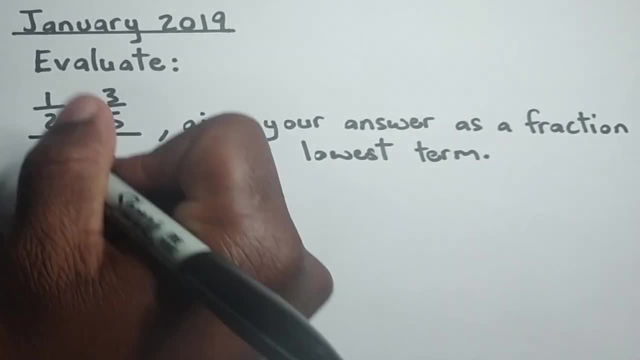 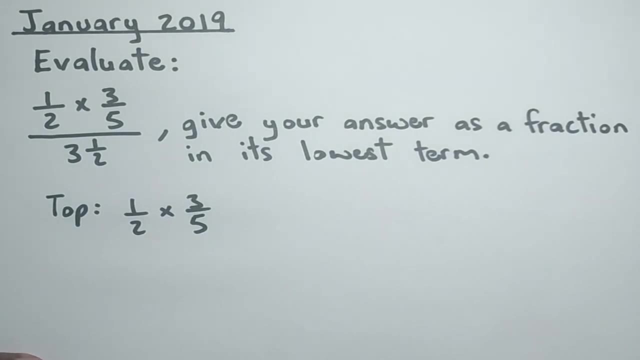 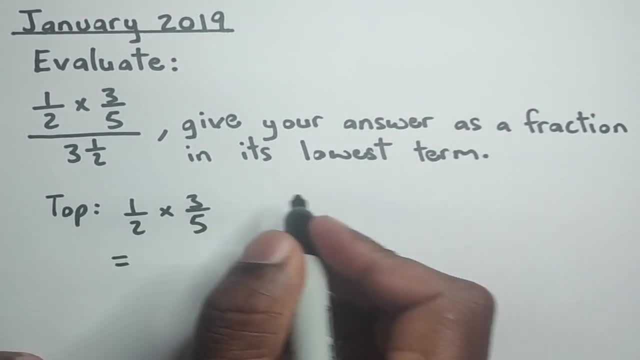 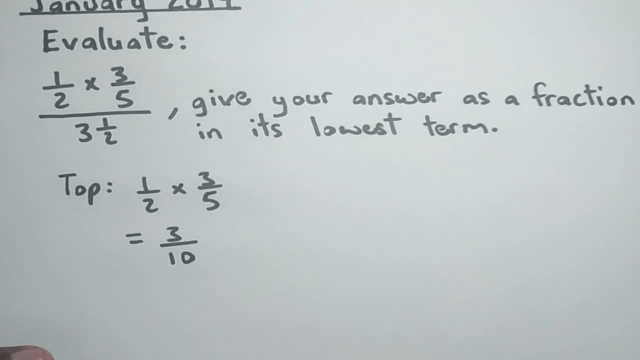 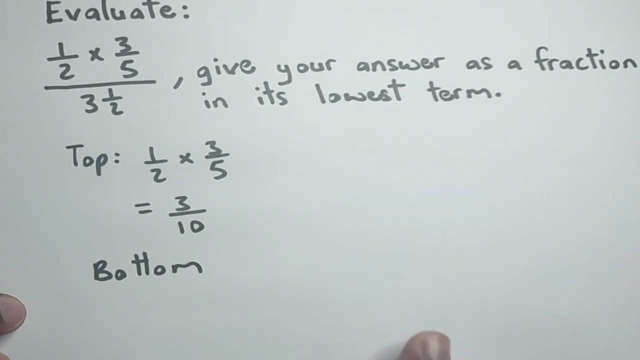 numerator and denominator by denominator. so one times three, that's three. two times five, that's ten. all right, and we're pretty much finished with the top now. here we have the denominator, we have the denominator to treat with now, and we're just going to convert this thing to an 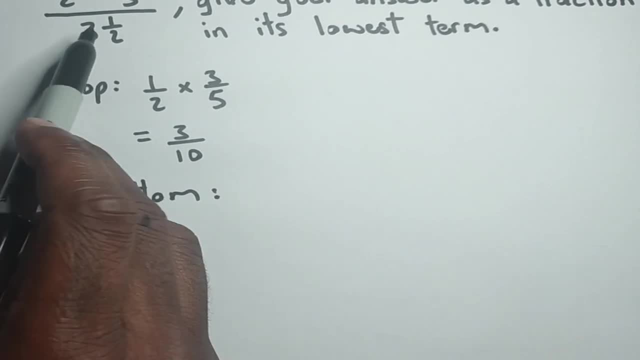 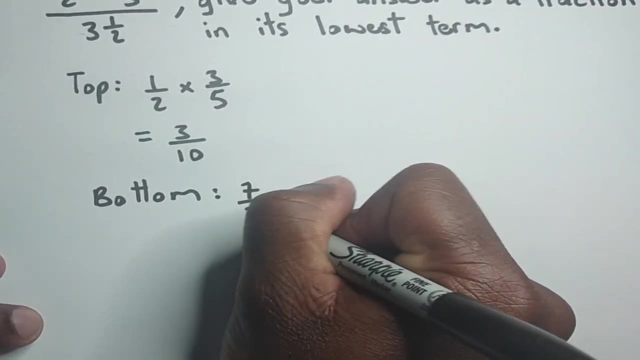 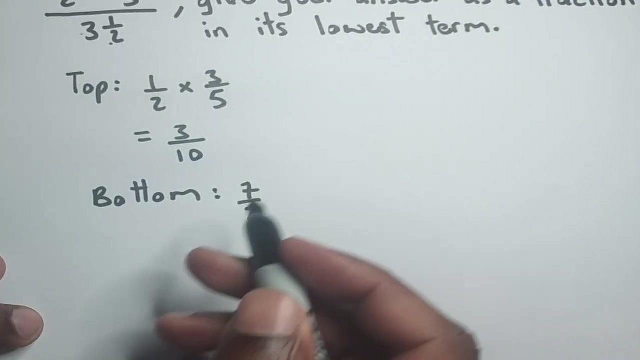 improper fraction. so three and one over two is the same thing as seven over two. all right, so three times two, that's six plus one, that's seven over two. so we'll multiply the whole number by the denominator and the result that we get we'll add that to the numerator. all right, so that's how i. 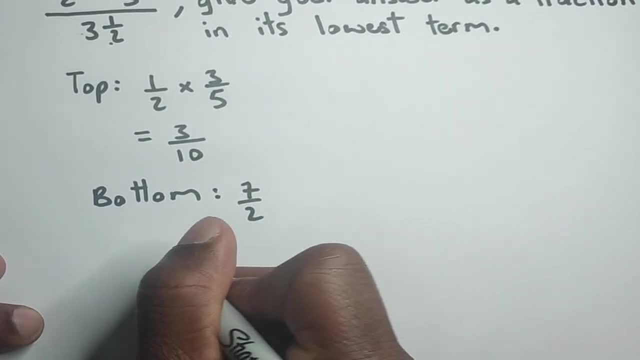 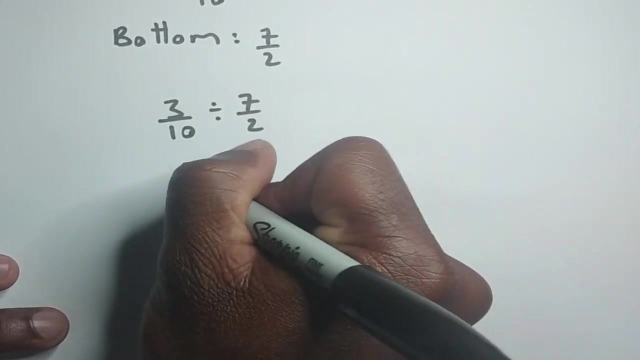 get this thing right. here and again, we'll divide the top by the bottom. so we have three over ten divided by seven over two. all right, and when we're dividing fractions, we keep the first fraction. so we'll keep the first fraction, which is three over ten. in this case, we change the sign. 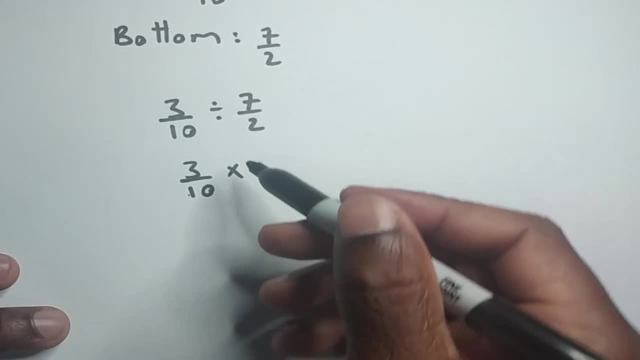 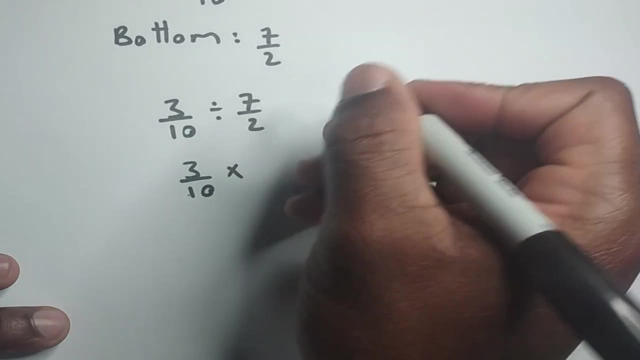 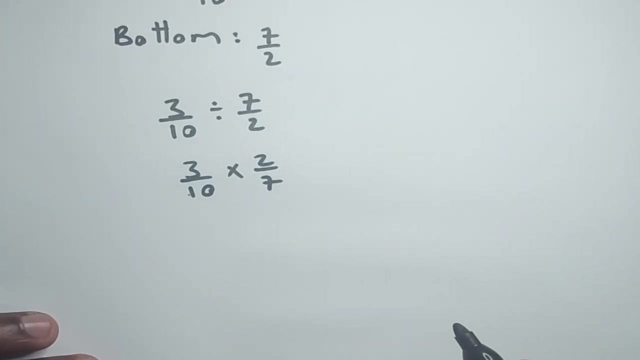 the division sign to multiplication, and then we'll flip the second fraction, which will refer to as the reciprocal. all right, which simply means that we're going to flip this thing. so seven over two will become two over seven. all right, and we can do some simplification right here, so we can simplify, so two into itself goes. 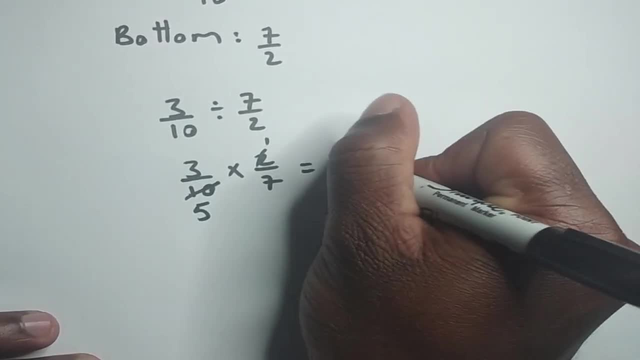 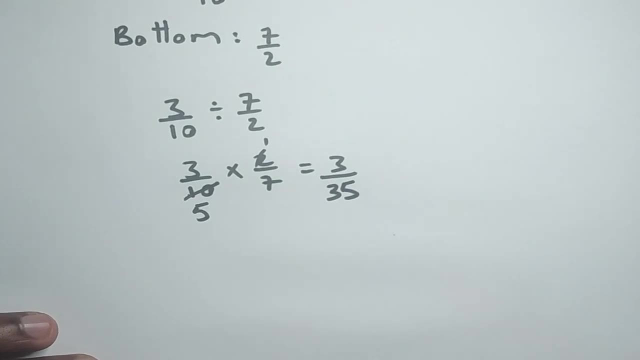 one. two into ten goes five three times one. that's three over five times seven, which is 35. all right, and this is pretty much our answer. so this is how we give our answer as a fraction in its lowest term. all right, and that's how we treat with this particular question. now, here we have general 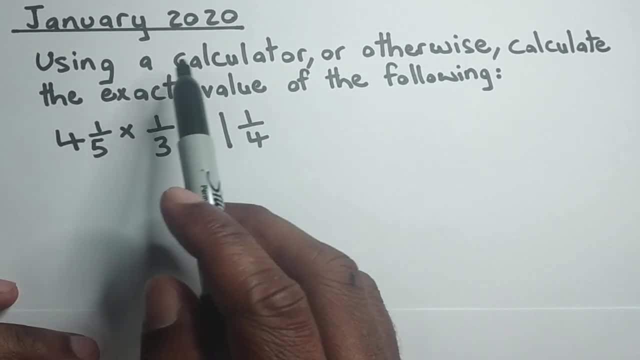 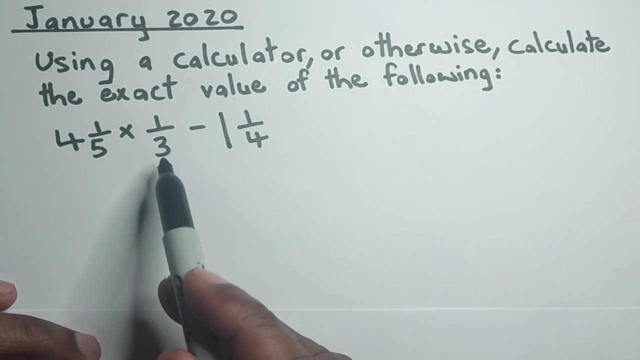 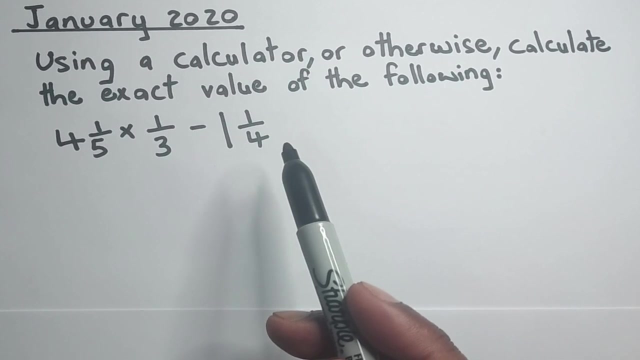 two thousand and twenty, all right. and this is us, using a calculator otherwise calculate the exact value of the following: four and one over five times one over three minus one and one over four, all right. so this is the most recent fractional question that was given on the csec exam, paper two. 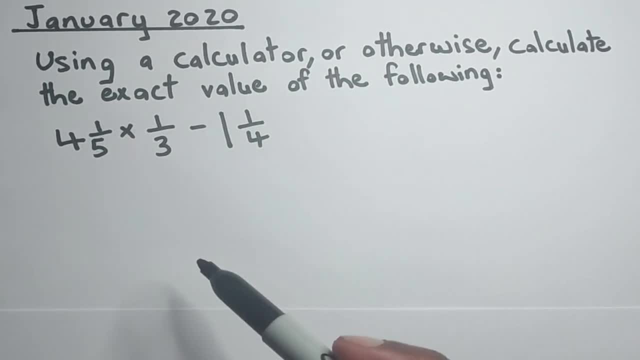 that is all right. and before i solve this question for you guys that are going to sit the june exam, you guys can let me know in the comment section which topics you would rather me to look at and the past csec papers, and i'll do so, all right. so what you guys can do, you can mention that down in. 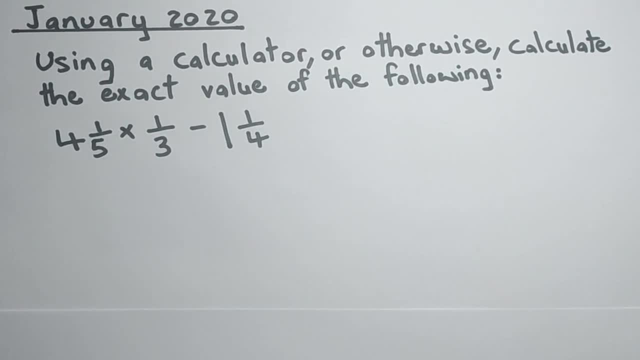 the comment section below and i'll look at those and, in short, i'll address those questions that you have down there. all right, so we have four and one over five times one over three, minus one and one over four. now what we are going to do is to convert the mixed function into the mixed function. 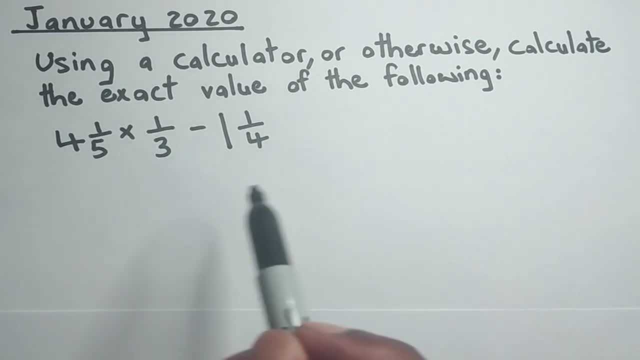 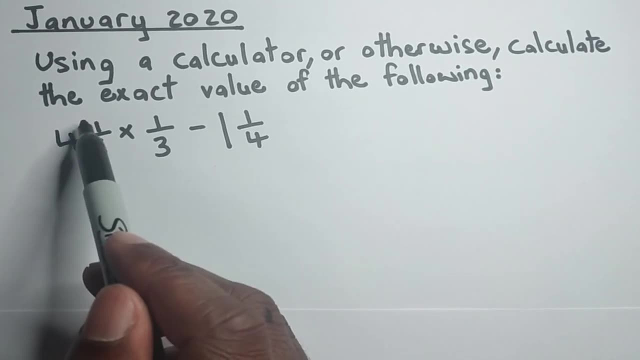 to improper fraction. all right, and we have two here, so four and one over five. again, we'll multiply the whole number by the denominator and then we'll add the result to the numerator. so four times five, that's 20 plus one, that's 21. so we have 21 and we keep the same denominator: 21 over five times one. 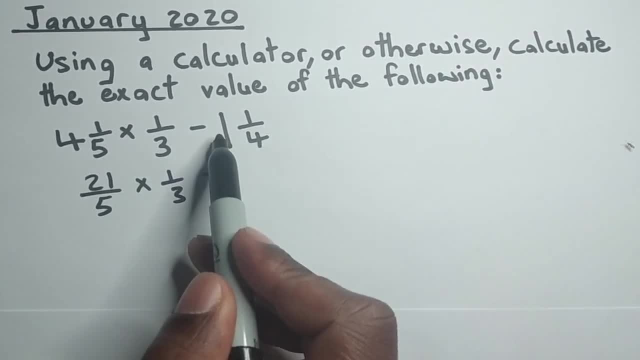 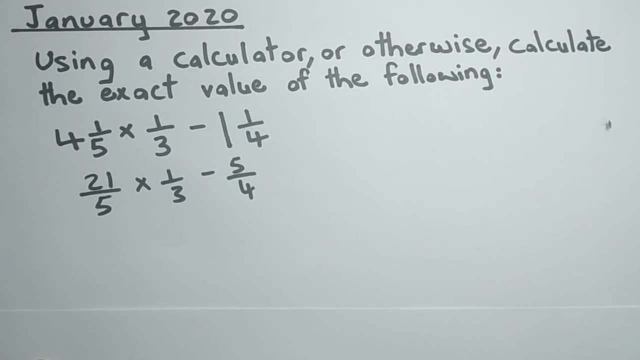 over three minus again, we do the same thing one times four. that's four plus one, that's five over five over four. all right, now what we're going to do? we have to multiply first because, according to the order of operations, we have to multiply before subtract. if you also want to learn the order of 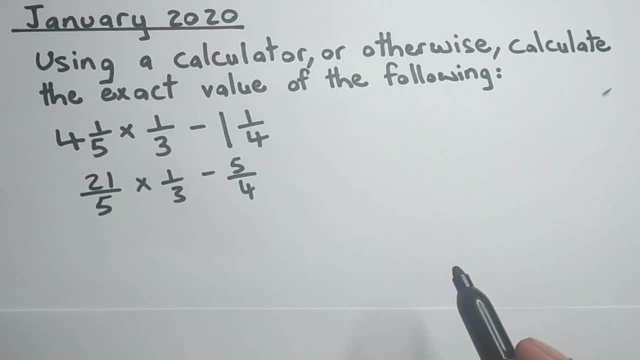 operations. you can check the description below. i'll have that video titled order of operation and the link to that video will be in the description section below. all right, so what we can do here we can cancel. so i'm going to put the multiplication section in bracket. so